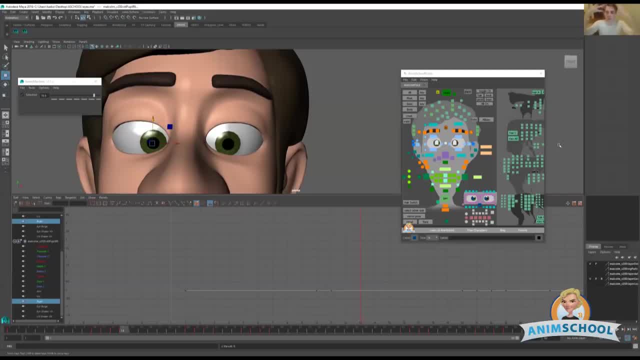 tend to contract because more light is hitting the surface And when we look down, we tend to block more light from the surface and the pupils expand. Likewise, when the lids come down over the eye, that blocks light from the surface of the pupil. 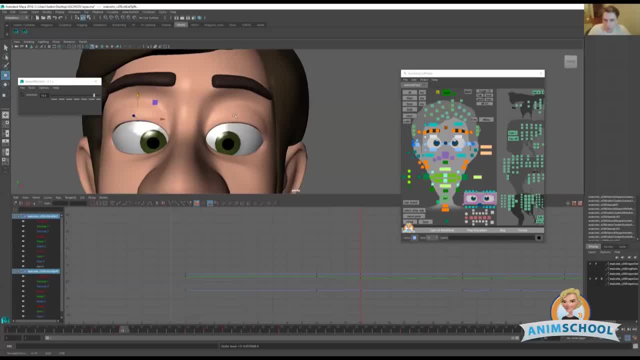 And the pupil tends to get bigger. And when the reverse happens, the pupil tends to get smaller. Easy enough to remember, right? So we start them a little bigger than normal, just a bit. not enough that he looks like he's on drugs of some sort, just a little. 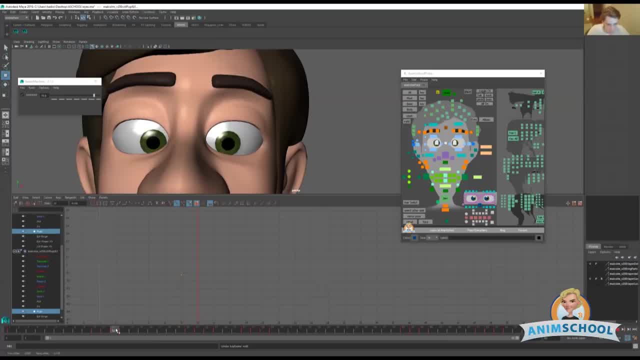 bigger than the default. And then, as this eye dart happens and the lids come down, they block some light from the sun or from the lights above or from the eye direction, from those pupils. going lower on that circular surface of the eye also makes it harder for the light. 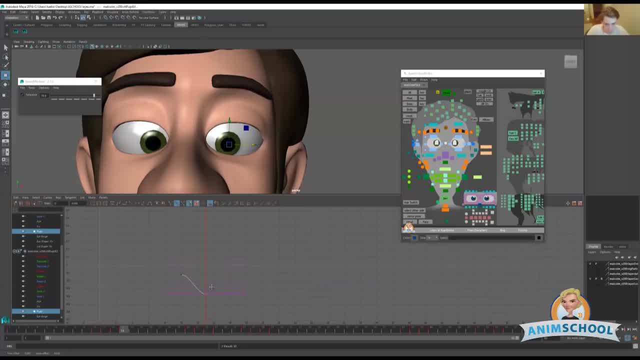 to reach them. So it's probably going to expand. Oh yeah, so I should make our opening one a little smaller actually, And then, as he looks down, they expand a little. that's too much, but then on an eye dart like this, 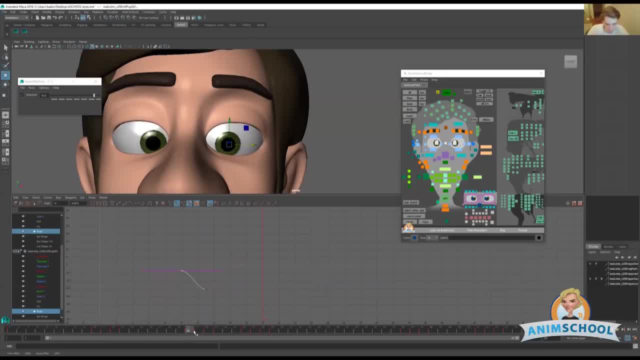 see how the upper lids coming down a bit, so I might take that information and, okay, across those three frames, as the upper lid comes down, I will increase that pupil size a little and what this does is starts to loosen up that pupil on close-up shots like this and make it feel alive just a little bit. you don't. 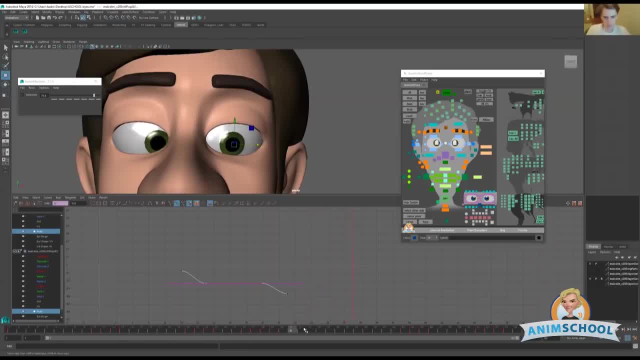 want it to feel like it's blooming or anything, and I'm probably overdoing it a little bit here. I'm just going to go through and animate for the rest of these eye dots. okay, let's see what that does. now look closely at those pupils.